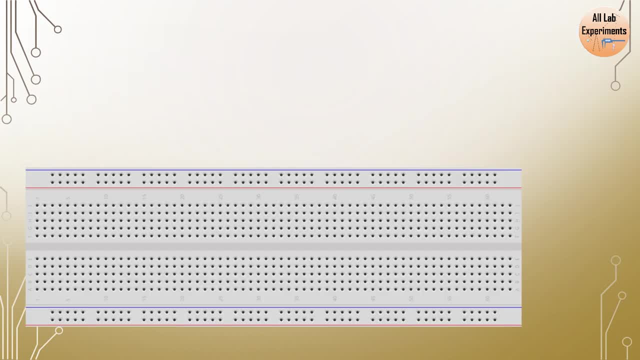 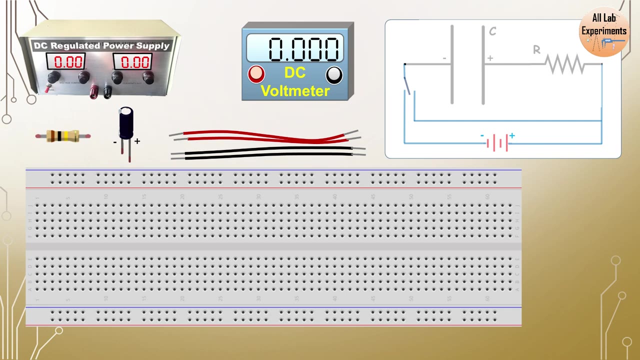 is done. To perform this experiment, we need a breadboard. Along with this, we need a power supply, a DC voltmeter, some components like a resistance and a capacitor and some connecting wires. And here is our circuit. Now, in the first step, we connect our power supply. 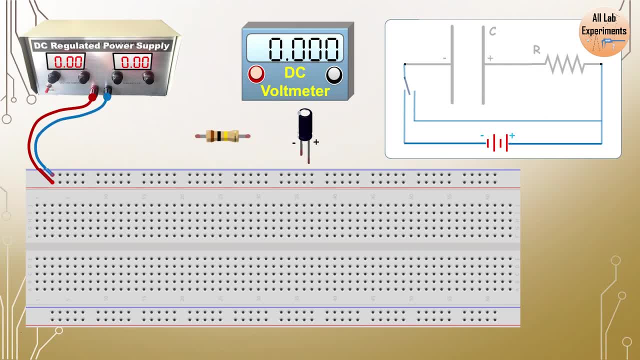 to the breadboards, to horizontal line on the top In the circuit. you can see that the battery and the connected wires, they have been highlighted. Before moving further in this experiment, I must tell you that choose the value of capacitance and resistance wisely, such that 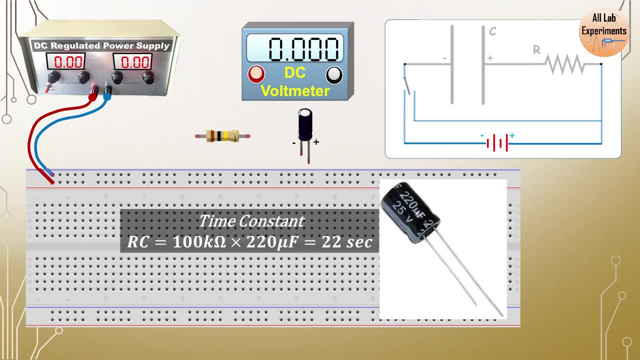 that the product of R and C should be a reasonable value. It should not be that small, like 2,, 4, 5 seconds, and it should not be that high, like 400, 500 seconds. In both cases, you will face trouble while observing its readings. So this is a good combination and you can choose. 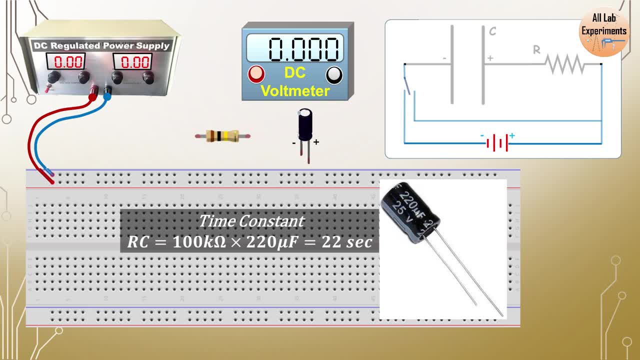 one like this or close to this. So I am choosing 100 kilo ohm resistance and 220 micro ohm capacitor. Also check what is written on your capacitor. So with 220 micro farad, you can see here it is. 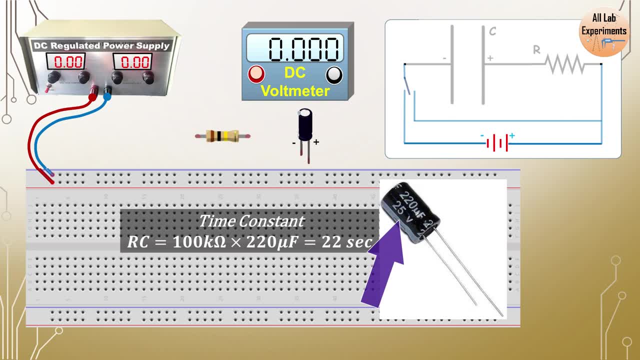 written: 25 volt. So 25 volt is the maximum voltage which this capacitor can bear. So don't apply any voltage higher than this in any part of the experiment. Just take care of that You need to take care. one more thing here: There could be some charge on this capacitor, So just take some. 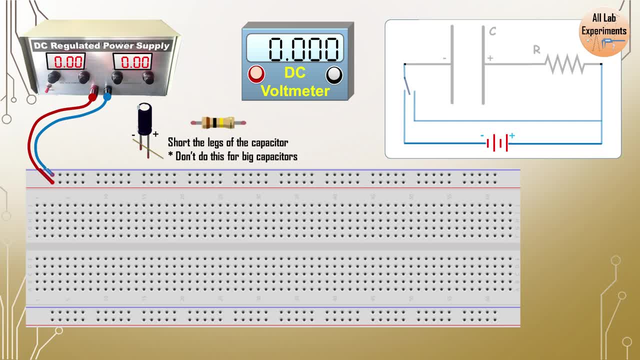 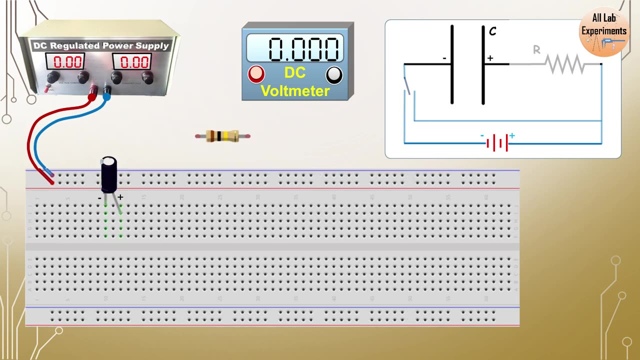 wire and short the legs of this capacitor. You can do this for this small capacitor, but don't do this for a big capacitor, because in that case you may see some sparks. Just insert the legs of this capacitor in the breadboard So we can see two vertical lines. They have been highlighted with. 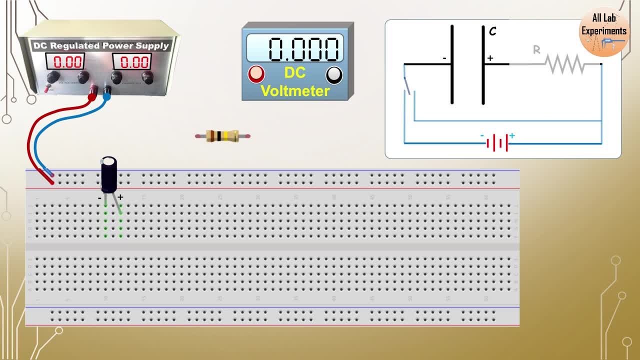 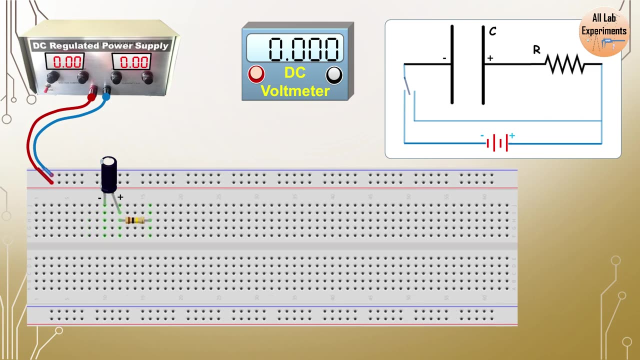 mild green color. in this and also in the diagram, you can see that there are two vertical lines, So you can see that this capacitor has been highlighted. Now, in the next step, we are going to connect this resistor in series with this capacitor, As we know that, vertically, these lines are connected. 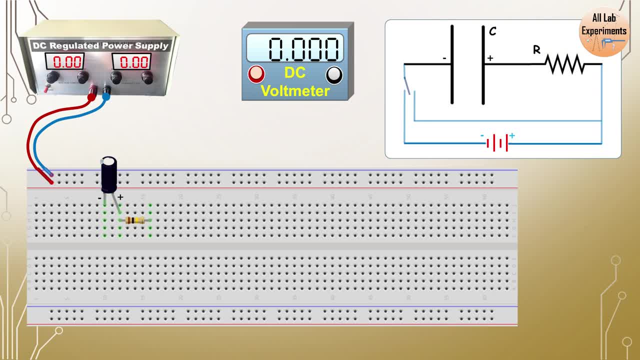 So we have placed one end of the resistor in the same vertical line in which we have already inserted the positive leg of the capacitor. Generally, we read in theory that capacitors don't have polarity, but one which we are using here. this capacitor has. 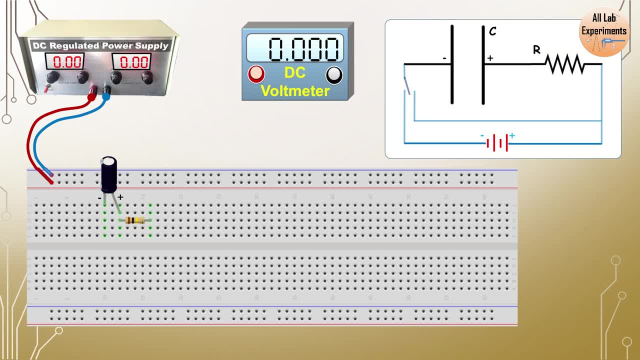 a polarity. So we are going to connect the positive of the battery to the positive of the capacitor, But we want to charge this capacitor through a resistance. So now we can connect this wire from the horizontal line in which we have already provided the positive leg of the capacitor. 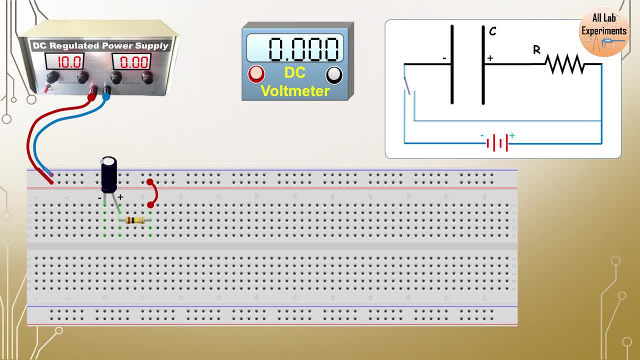 So this capacitor has already Attack Power empresa, So this capacitor has fire smell, so we are going to connect this wire. Let me show you a very easy way to complete this loop. So we have already provided 10V using the regulated power supply. 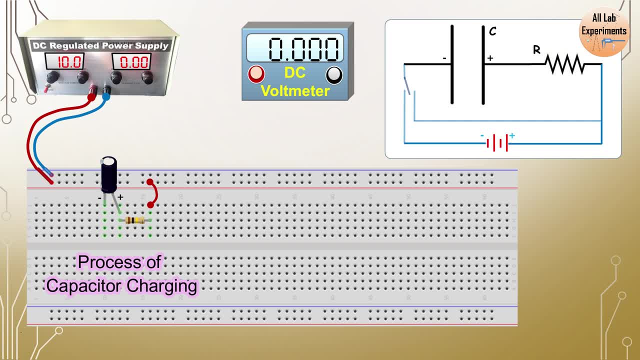 From that we have connected one side of the resistor Again, we can match this with the circuit diagram. Just the time when we complete this loop, This capacitor will start charging. So we need to take readings from that point only. So, before that. 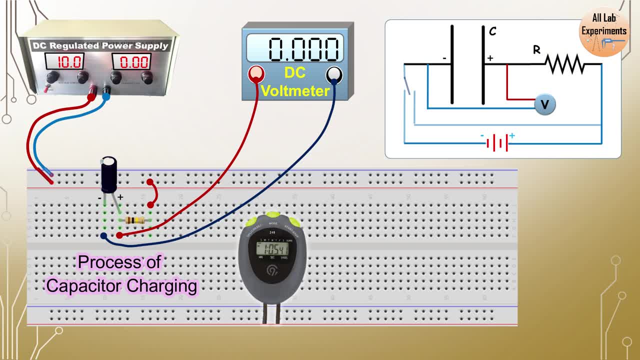 we are going to connect, take a stopwatch, be ready with that and finally connect the negative leg of the capacitor with the negative of the battery. so just the time you complete this circuit, this capacitor will start charging and you can observe the voltage developed across this capacitor in. 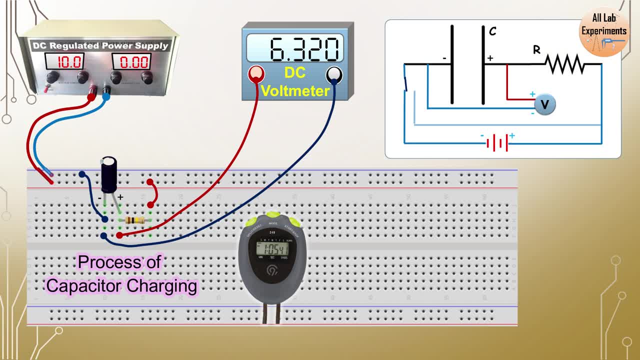 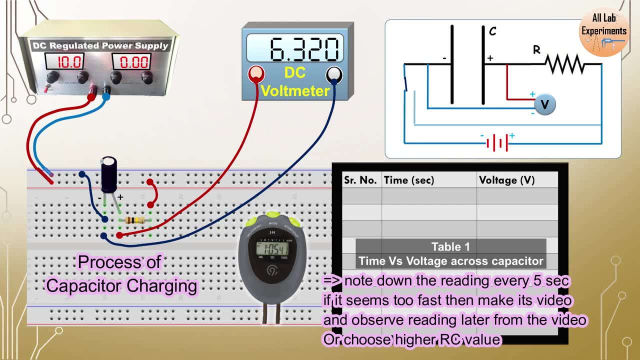 this DC voltmeter now make the first table. in this table you are going to note down the voltage developed reading along with the time. so just take note of that and that's it. so voltage will reach a maximum value if you have applied 10 volts, so close to 10 volt. 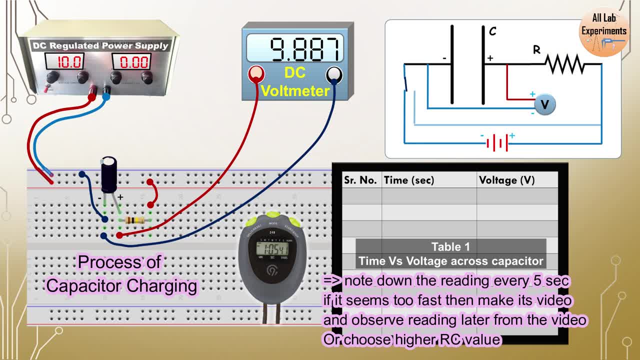 this voltage will stop increasing at that point. so you have finished one part of this experiment in which you are charging the capacitor. now you can start the second part of this experiment in which we are discharging this capacitor. first we disconnect the battery, so we removed this positive and negative wires. now we will. 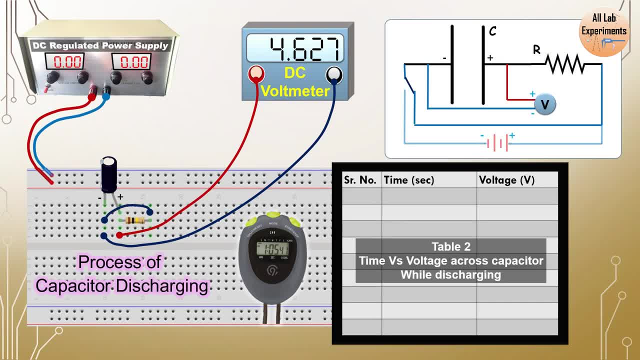 connect the negative of our capacitor with the other part of the resistor. the negative charges from one part of the capacitor are moving to the other plate, but in between we have this resistance. you can also observe this in the circuit. the highlighted part only is now on the breadboard. 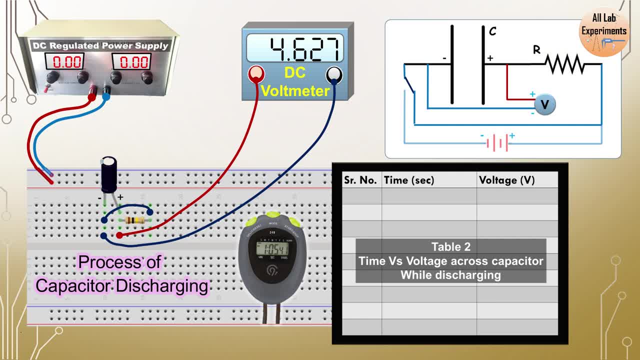 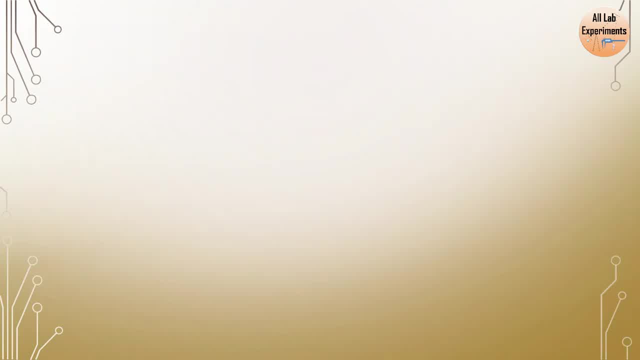 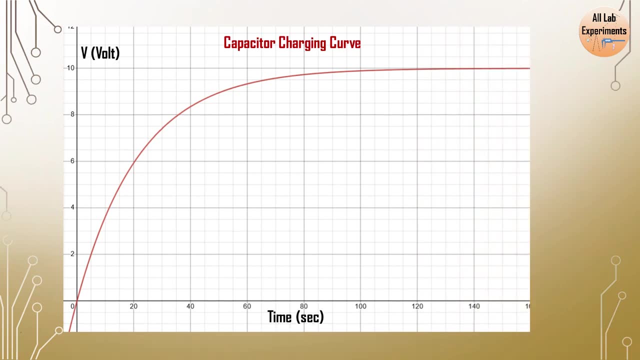 just reconnect the wire, so this capacitor started discharging and we are going to observe this in the table too. now further experiment is also quite easy. just take time on the x-axis and voltage on the y-axis and plot this curve. by definition, the RC time constant is the 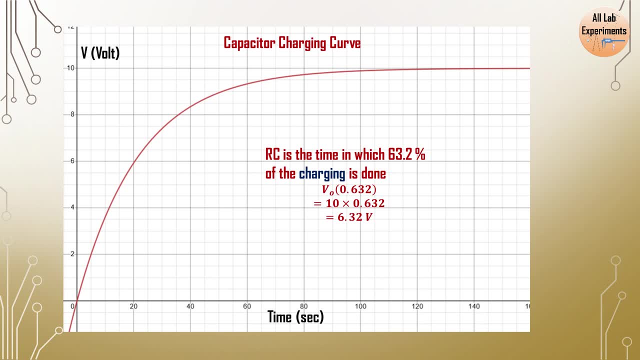 time in which 63.2% of the charging is done. it means if you have applied 10 volt potential difference across your capacitor, so 6.32 volt potential difference will be developed in one RC time. so just we pick this point: 6.32 volt and corresponding. 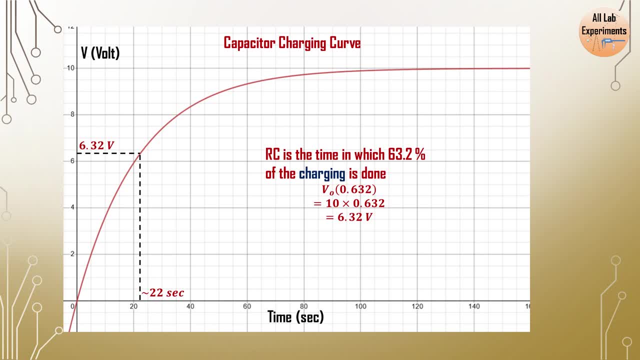 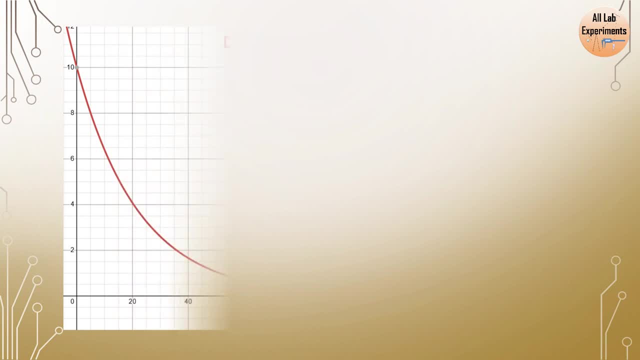 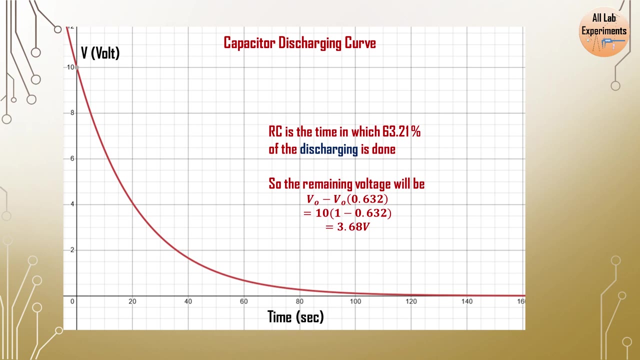 to that voltage. we observe the time, so this is close to 22 seconds which we have taken in our example. in the same way we are going to plot capacitor discharging curve. by definition, RC is a time in which 63.21% of discharging is done. we can imagine that out of 10 only. 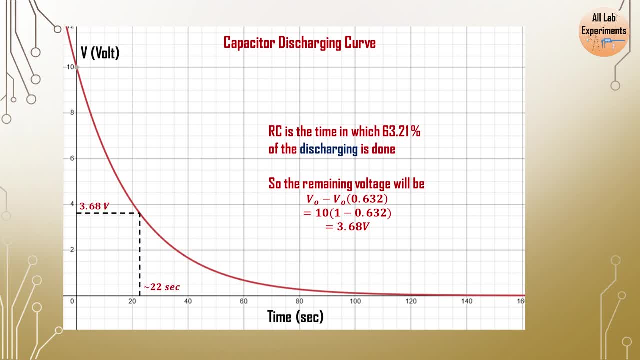 3.68 volt will be remaining. find the time corresponding to that as well. this is your time constant observed from charging and discharging curves. now, as a final calculation, we know that theoretical time constant is 100 kilo ohm into 220 micro farad is equal.